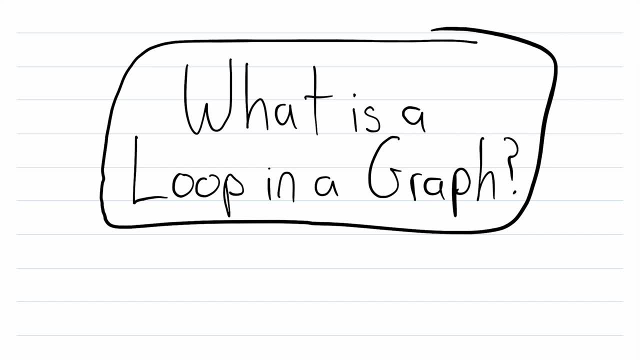 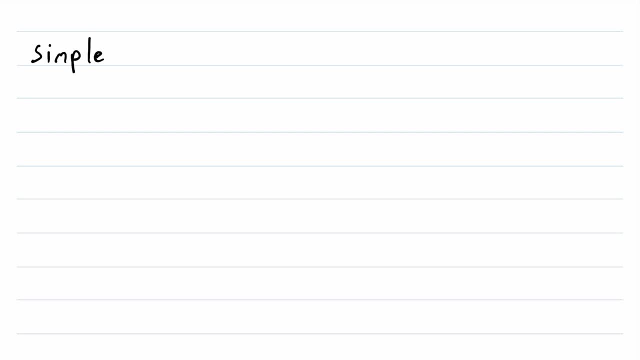 to have, but I'm going to try to keep this lesson as much of a general overview as possible. So, with that said, let's get into the lesson. Usually, when we begin studying graph theory, we spend most of our time studying what are sometimes called simple graphs You're probably familiar with. 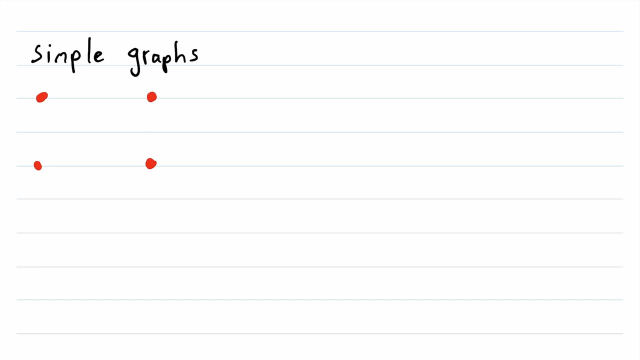 simple graphs. They've got vertices and they've got edges that join pairs of distinct vertices. There are a few things that simple graphs are not allowed to have. For example, in a simple graph, a pair of vertices is either joined by zero edges or one edge. They're not allowed to be joined by. 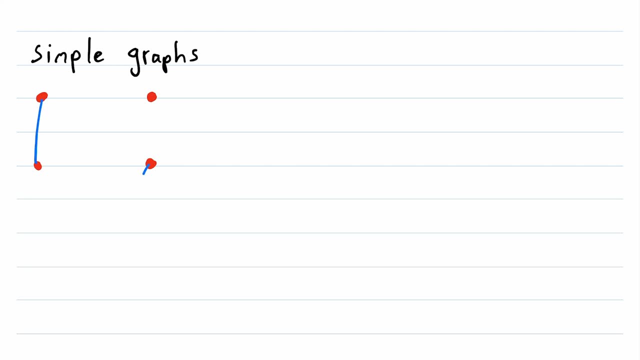 more than one edge. Also, in a simple graph, an edge is not allowed to join a vertex to itself. And let's stop there, because this is what's called a loop. So again, a loop, also sometimes called a self. 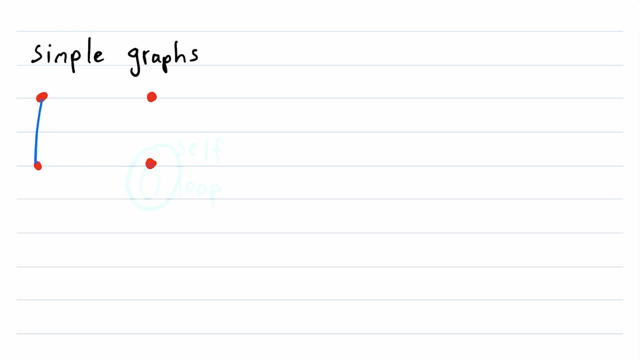 A self loop is an edge that joins a vertex to itself. And again, loops are not allowed in simple graphs. So if you are using vertices to represent people, and let's say you are using edges to represent friendships between those people, then a simple graph will do just fine. It wouldn't make sense to 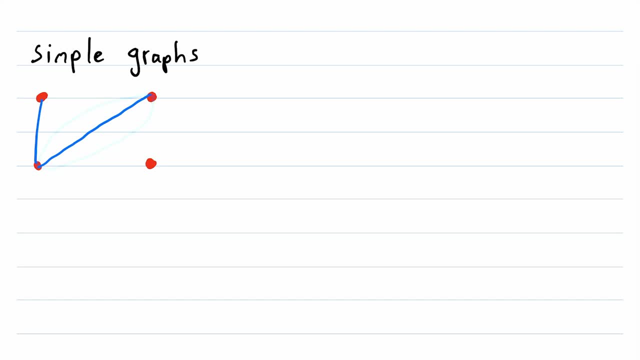 have multiple edges between the same pair of vertices, and it wouldn't make sense to have an edge joining a vertex to itself, because you can't be friends with yourself. But what if we change people who have the same age? So then, if this vertex down here is Alex and this one over here? 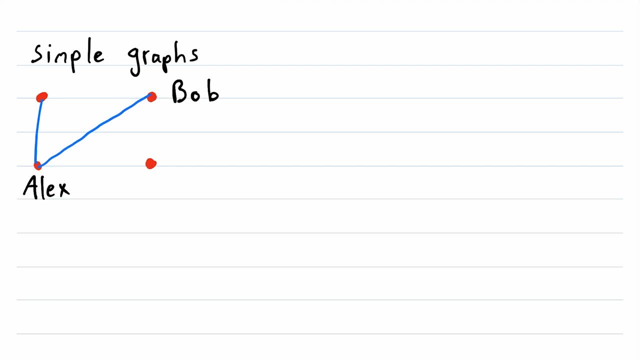 is Bob. this edge between them means that Alex has the same age as Bob. Now, in this case, it would make sense for an edge to join a vertex to itself, because everybody is the same age as themselves. We could, of course, just choose to not include these edges, but again, if we do, these are loops. 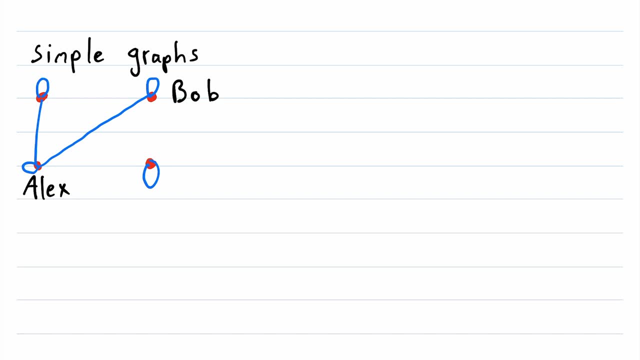 edges that join a vertex to itself, And this is a big part of what math is all about: that curiosity to take something that we previously didn't allow, like loops, then allow it and see what happens. An interesting question to ask now is: what is the degree of this vertex? Remember? 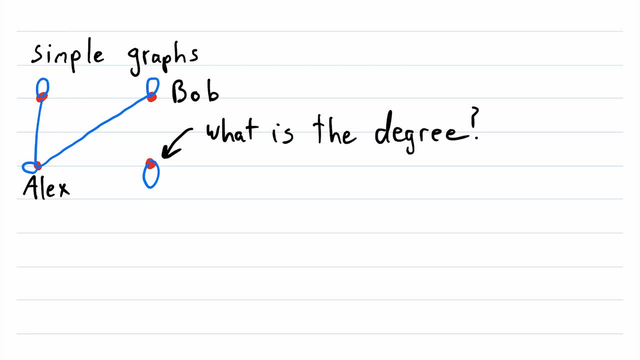 that in simple graphs we said that the degree of a vertex is the number of vertices it's adjacent to or the number of edges it's incident to. So you might be tempted to say that the degree of this vertex is the number of vertices it's adjacent to or the number of edges it's incident to. 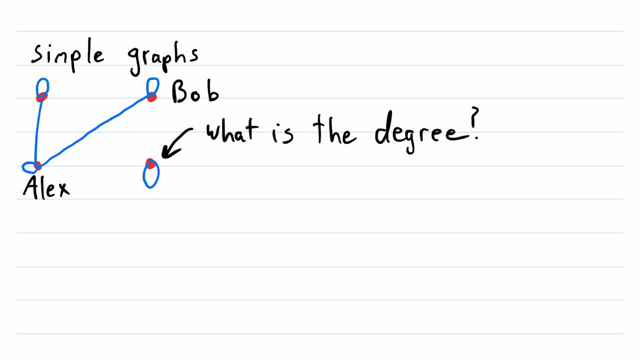 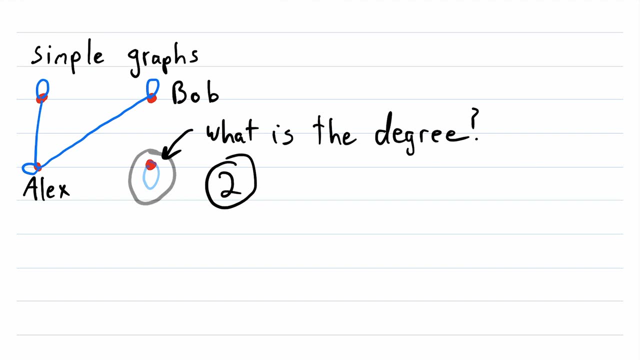 it's only adjacent to itself, but in fact its degree is two. You could think of this as being because an edge contacts this vertex two times. If we draw this loop again, you can see the edge contacts the vertex once and then it comes around and contacts it a second time. So that's one way. 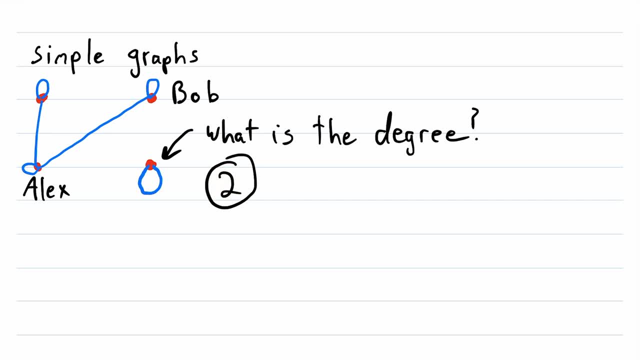 of justifying this, that the degree is two. One of the benefits of loops contributing two to the degree of a vertex is that it preserves the first theorem of graph theory, which you might remember, that this function in the class is a constant and it's a constant in the class. So that's. 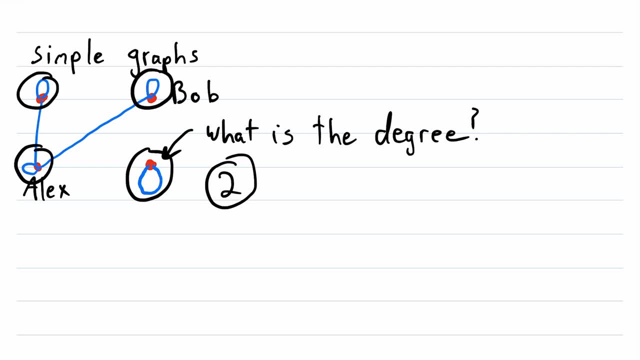 us. if we add up the degrees of all of the vertices in a graph, it will be equal to 2 times the number of edges. So just remember that loops contribute 2 to the degree of a vertex. So the degree of this vertex is 2, the degree of this vertex is. 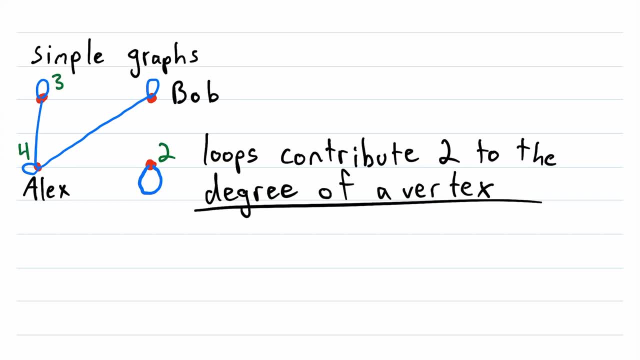 4,, the degree of this vertex is 3, and the degree of this vertex is 3.. Now let me just relabel these two vertices here. for the next part, We'll label this one A and this one B. Recall that with simple graphs we defined edges to be two. 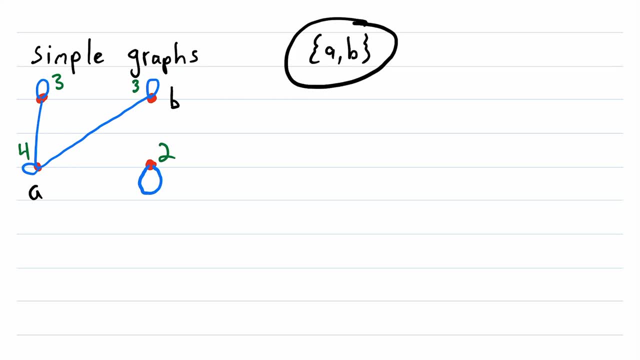 element subsets of the vertex set. So this is a formal representation of this edge that joins A and B. Now notice that using normal sets like this for a loop could cause some confusion, because the repetition of elements in a set does not matter, So this is just equal to this. Now I've seen a couple of definitions to get. 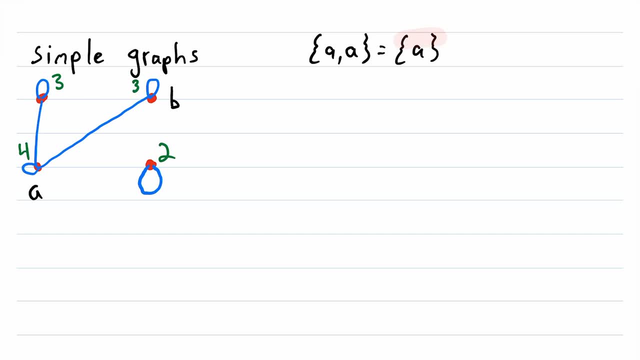 around this problem. The first solution is to just embrace it and simplify it. So I'm going to go ahead and do that. So I'm going to go ahead and say that this is what a loop is. It's a one element subset of the vertex set. So if 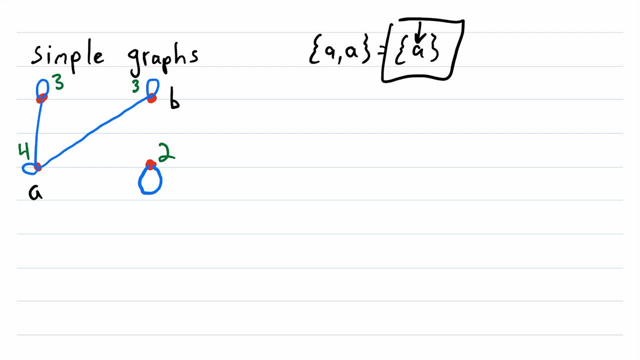 one of these elements of the edge set only has a single vertex in it. you know that represents a loop. The other solution I've seen is to use multisets instead of traditional sets. Multisets are just like normal sets: they're unordered. 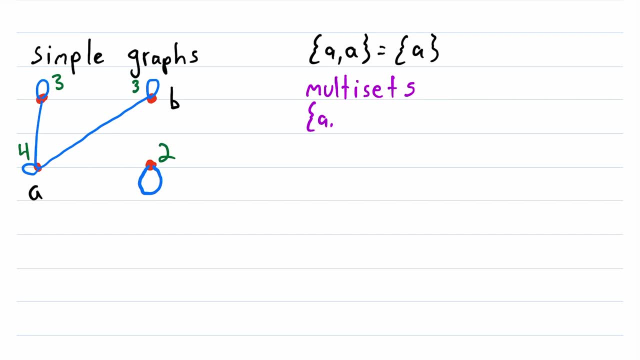 collections of objects, except for the distinction that they count multiplicity. So this is a multiset with two copies of the vertex A and this is a multiset with one copy of the vertex A, and as multisets they are not equal. Multisets are also sometimes.